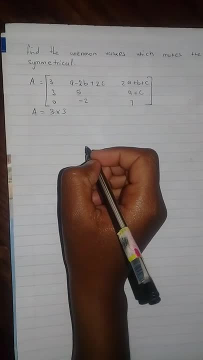 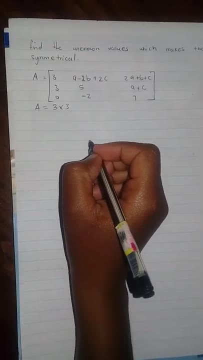 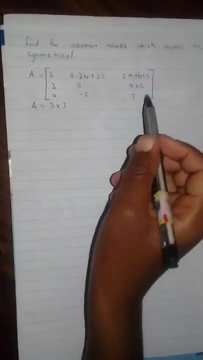 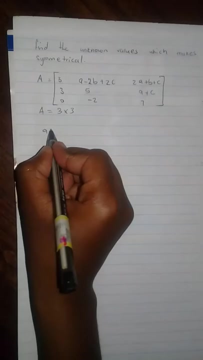 a symmetrical matrix will give you the values which are the same going forward and the same going backward. By that I mean okay, for example, let's just do it This- I'm going to start with this part because it seems less complicated: A plus C. this is in row one, two, three. 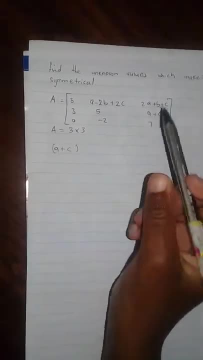 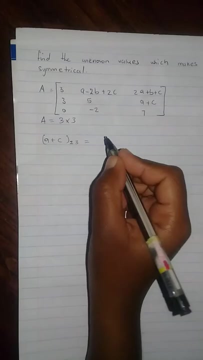 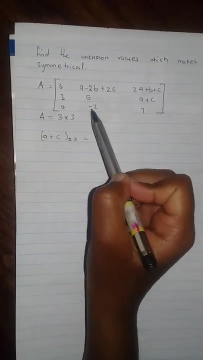 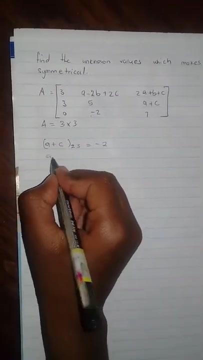 So this is row two, column one, two, three. So this is row two, column three. It must be the same to the value in row three. one, two, three, column two, one, two. So here it must be equal to negative two. A plus C is equal to negative two. That is my equation. 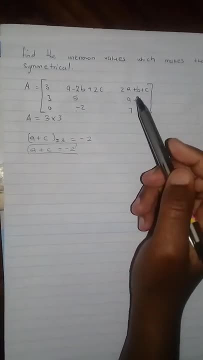 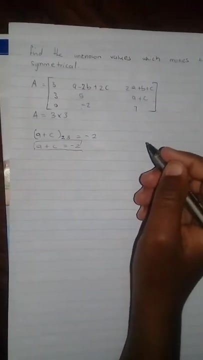 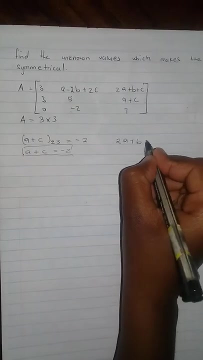 One. We go again to this part. Remember, you can choose Echo to go with this, this or that, But in this case I started with this because it seemed less complicated to me. We go to 2 a plus b plus c. this is in. 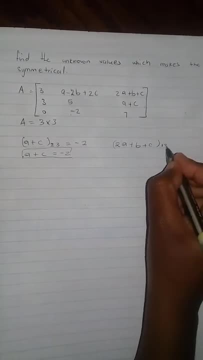 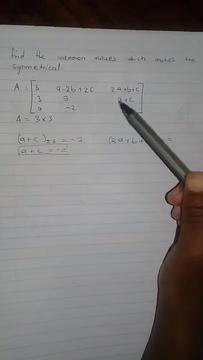 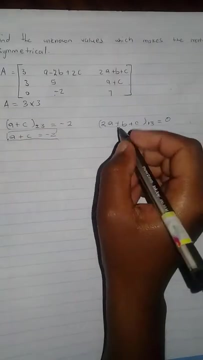 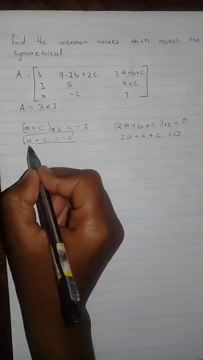 Row one, column three. It must be the same as the value in row 3: 1, 2, 3 kilo more 1, 2. so kilo minus 0 is equal to 0. so 2 a plus B plus C is equal to 0. here I make, you can choose. let's make C will aid the. 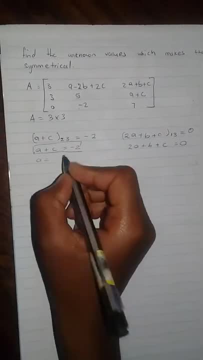 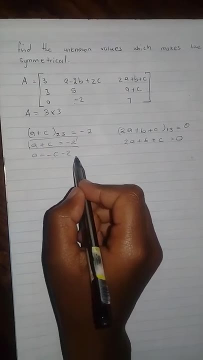 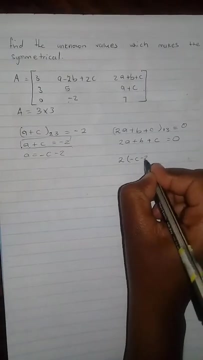 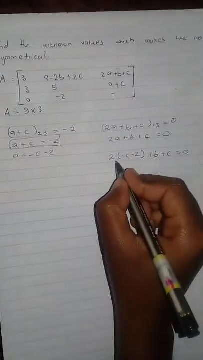 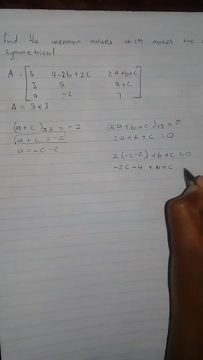 subject of the formula, but I'm going to choose to make a, because 2 minus C minus 2, so a is equals to minus C minus 2. come in the side 2. this is a minus C minus 2 plus B plus C is equals to 0. so this is minus 2 C minus 4 plus B plus C is. 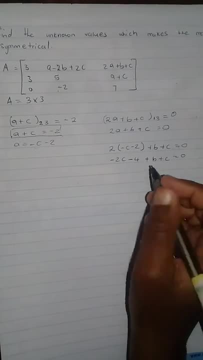 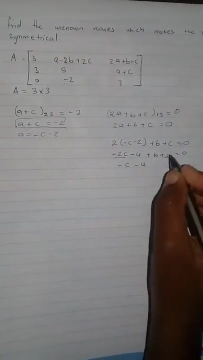 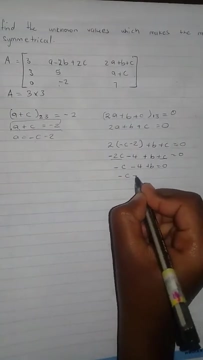 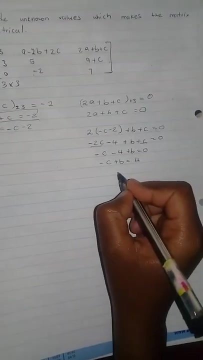 equals to 0. you have like times is 0, this and this. so minus C minus 4 plus B. because you 0 minus C plus B is equals to 4, you can add a choose again to make. C will be the subject of the formula I'm. 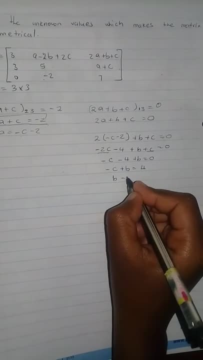 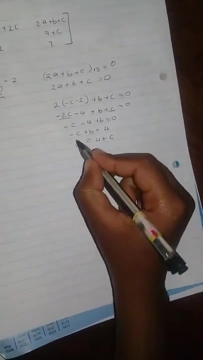 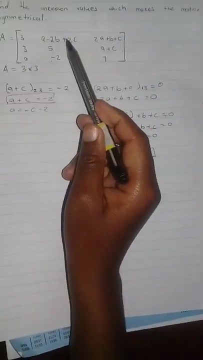 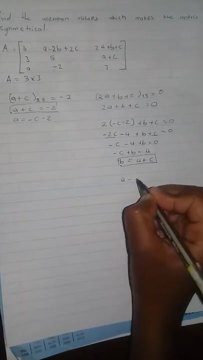 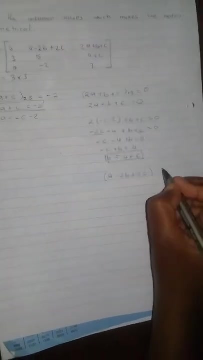 going to choose. B is equals to 4 plus C. this is my second equation. I will again go to this, this part, because I've already done. this is now next stop: 1 a minus 2 B plus 2 C. how do we label this? is in row 1, helium 2. this is my second equation. again. go to this this part, because I've already done. this is now a minus 2 b plus 2 C, leveled out as well, is in row 1, kilo 2. total: less than minus 2b plus 2c. this is in row 1, kilo 2. thank you so much for watching. this is in row 1, kilo 2, and I will see you in the next video, HELLO. 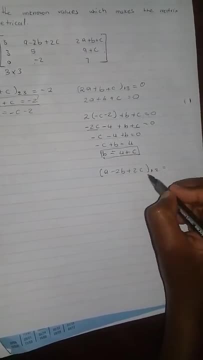 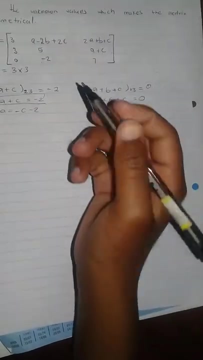 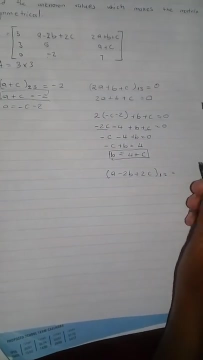 For the matrix to be symmetrical, this must be equal to the value in root 2, kilom 1.. So let's go to root 2, 1, 2, kilom 1, 3 here. So we see we have 3.. 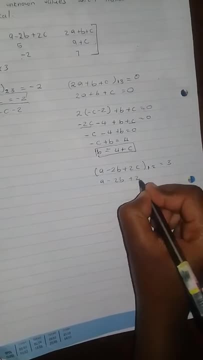 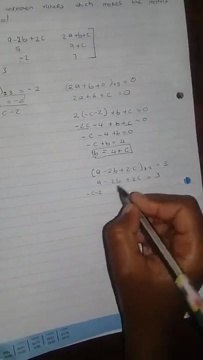 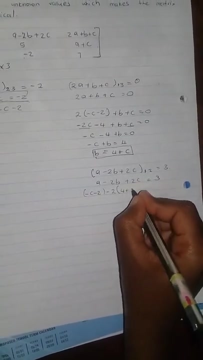 a minus 2b plus 2c is equal to 3.. Our a: we know we have it already: minus a minus 2, minus 2.. Our b: we have it here: 4 plus c plus 2c is equal to 3.. 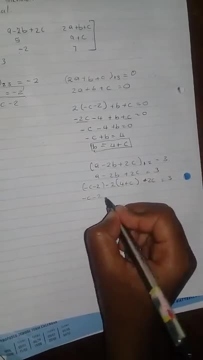 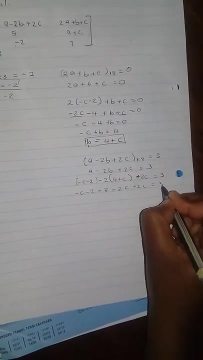 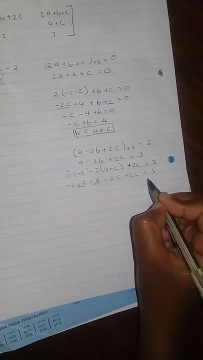 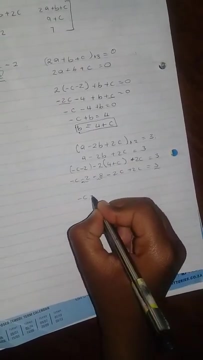 Okay, simplify: minus c minus 2, minus 8, minus 2c plus 2c is equal to 3.. Like times together: 2, minus 8, and 3.. Okay, minus c minus 2c plus 2c, we see something. 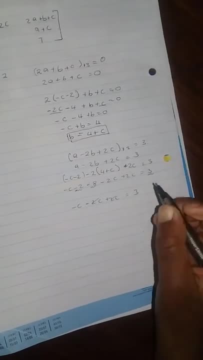 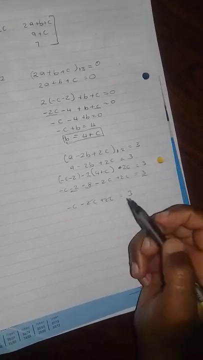 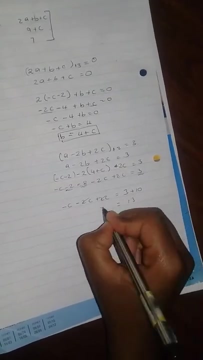 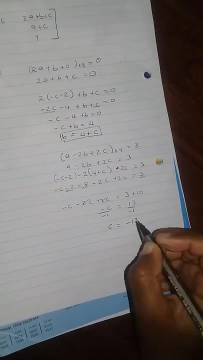 This will cancel out this. This equals to 3, minus 8, minus 2,. they give me minus 10.. Taking them to the other side, it will be positive 3.. So this is 13, minus c divided by negative 1, divided by negative 1, c is equal to negative 13.. 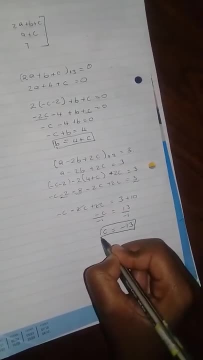 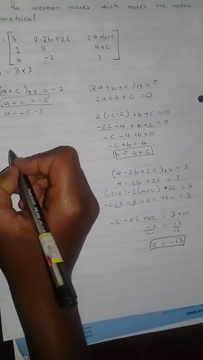 We now have the value of c. I'm sorry, I don't have enough space, So I'm just going to go ahead and use this. I hope you don't get confused. We have our c. We can find b, because we already have everything. 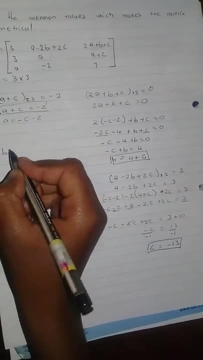 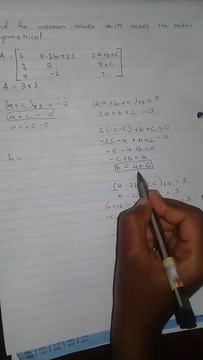 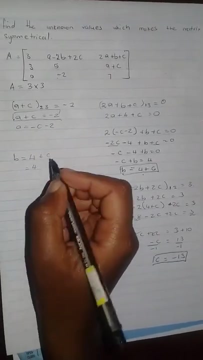 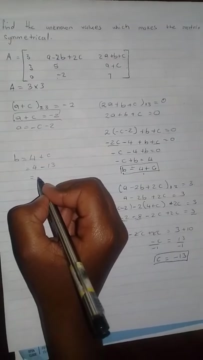 b is equal to. this is from this part where I made b. the subject of the formula is equal to 4 plus c. our 4. c is negative 13,. so 4 minus 13.. Okay, you do it on your calculator. 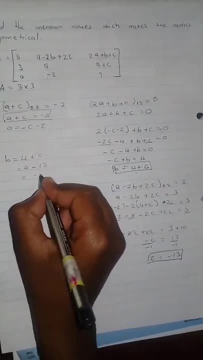 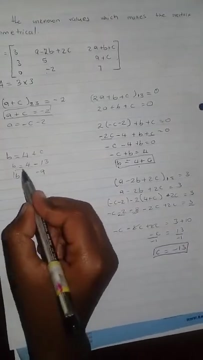 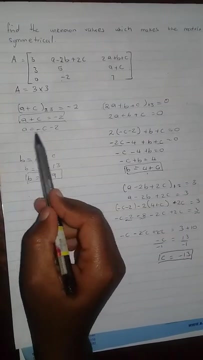 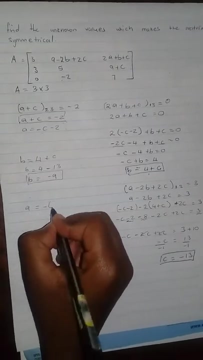 You get Minus 9.. This is it I have. b is equal to minus 9.. Now I go to c. That's our first equation, the one that we started working with. a is equal to minus. we know c is 13.. 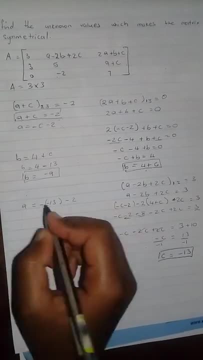 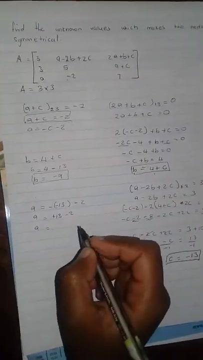 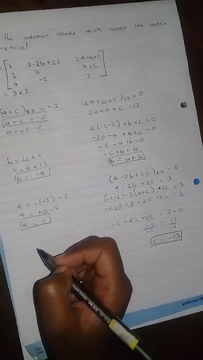 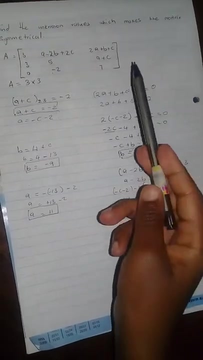 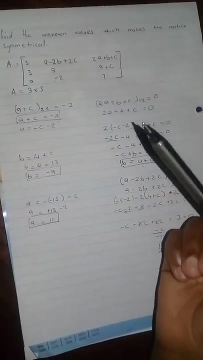 We know c is minus 13, minus 2.. This will be Positive 13 minus 2, so a is equal to positive 11.. So now we have the value of a, b and c. What we can do, we will substitute everything in the equations here in the matrix to get the values and verify that indeed this matrix is symmetrical. 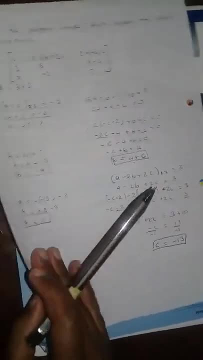 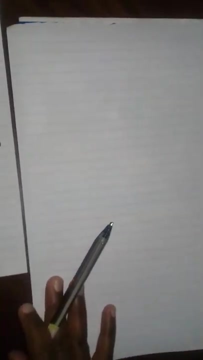 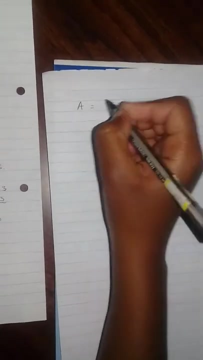 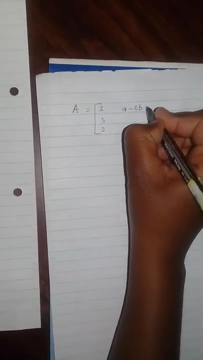 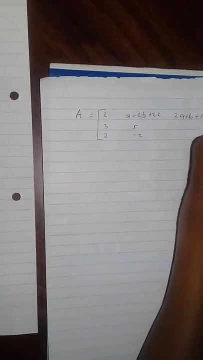 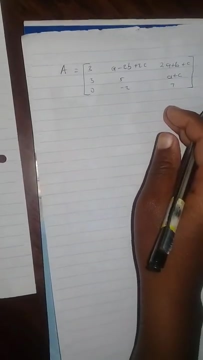 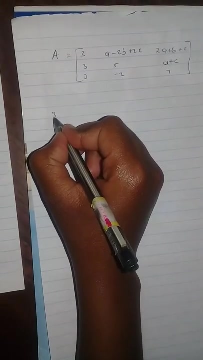 I'm going to need a new page, Okay. So our matrix, Go click on. write this again here: 1., 10. 60. 25. 22.. okay, so this is what we had initially then, because we know that three we know: 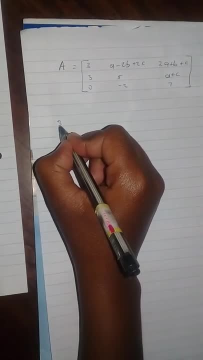 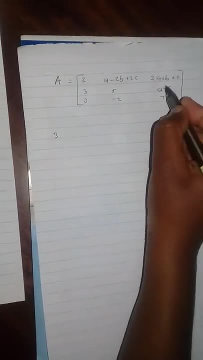 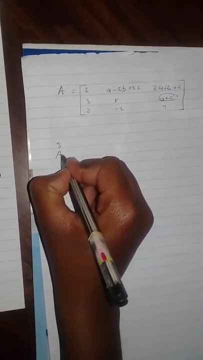 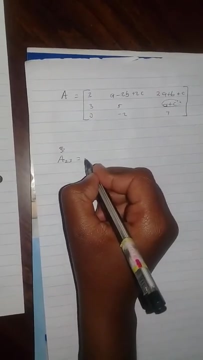 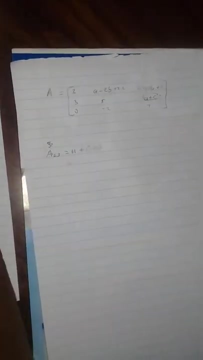 that value of C is a negative 13, B is negative 9, a is 11. what I'm gonna start with this part again. a to 3 to 3. a to 3 is a pussy. my a is 11 plus C is native pity. so that really day gives me. 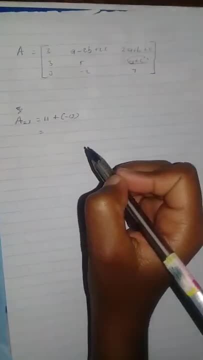 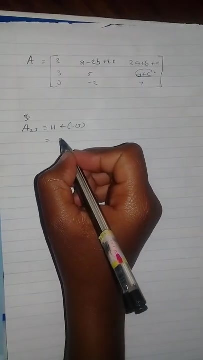 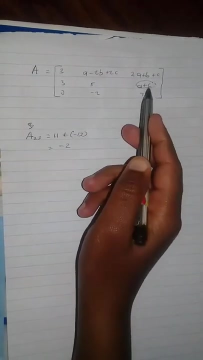 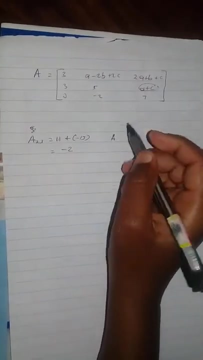 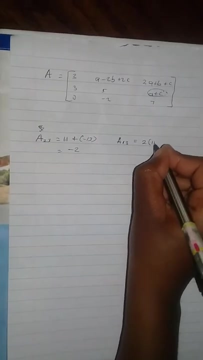 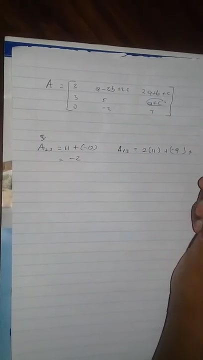 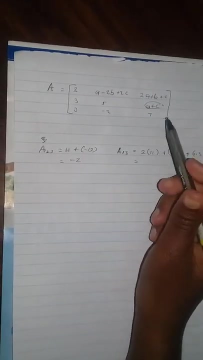 okay, this value here, 11 plus 13, it's gonna give me negative 2. so that part will be negative 2. we go again to a is because to rule 1, Ceylon 3 is a question, and to my a was 11, B was negative 9, C was native 18. so that's what all you mean do. 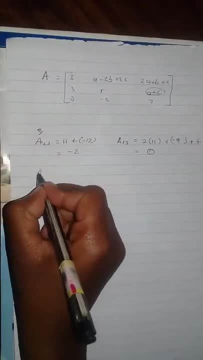 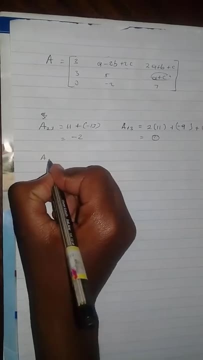 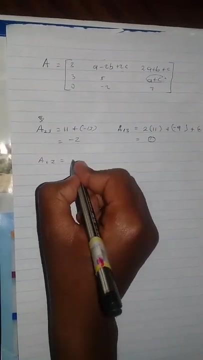 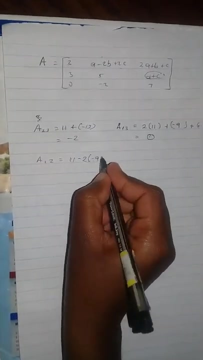 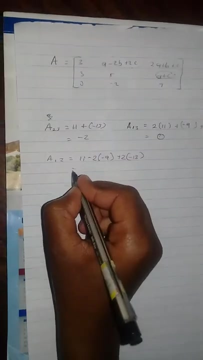 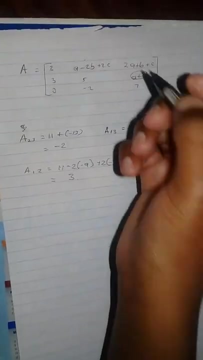 it on your calculator, you can get 0. a. there's fill here as it goes to rule 1: kill him too. a was 11 minus 2. our B was negative, 9 plus 2. C is native 13. you do it on your calculator, you're gonna get 3. so we see that this here is 3 and this. 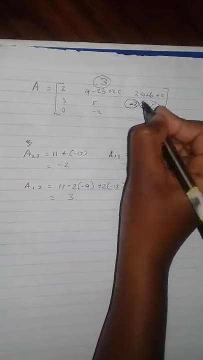 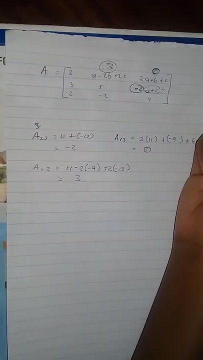 here is negative 9 plus 2. so that's what all you mean. do it on your calculator. you can get 0. a there's fill here as it goes to rule 1. C is a question. here is negative 2 and this here is 0. so removing all this, you're gonna get. 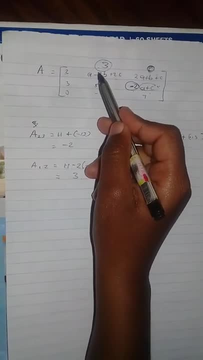 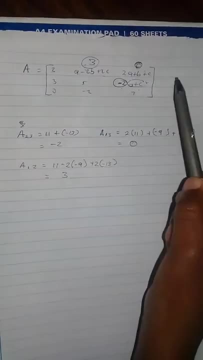 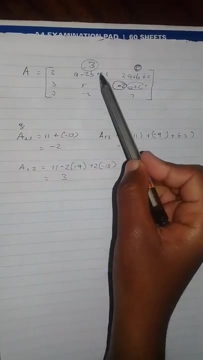 negative: 2, 0 and 3, which are equal when you go back and forward. if you want to see it, when you go to a row one, kill him too. a row one: kill him too. row one: kill them two. we get this if you go to row two. 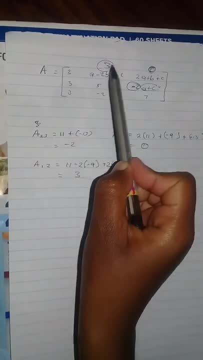 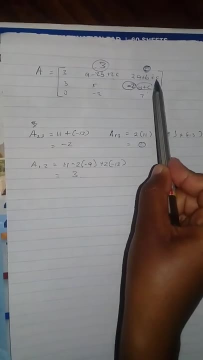 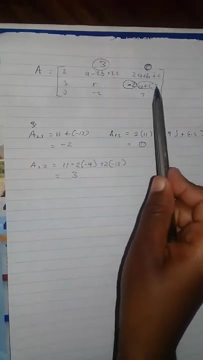 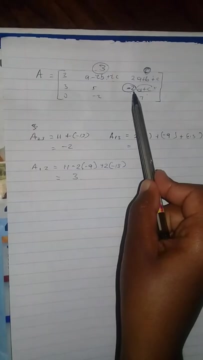 kill them one, you still get three. so this is a question that if you go again to row one, kill them three, you get zero. row three: kill them one, you get zero again. for this one, it's row two. kill them three, you get negative two. row three: kill them two, you. 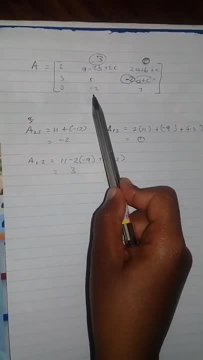 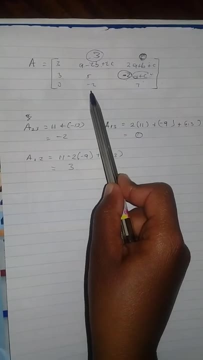 get negative two. so yes, the solution is symmetric. the matrix is symmetrical in the values, the unknown values, which makes um the matrix symmetrical as three: zero and negative two. 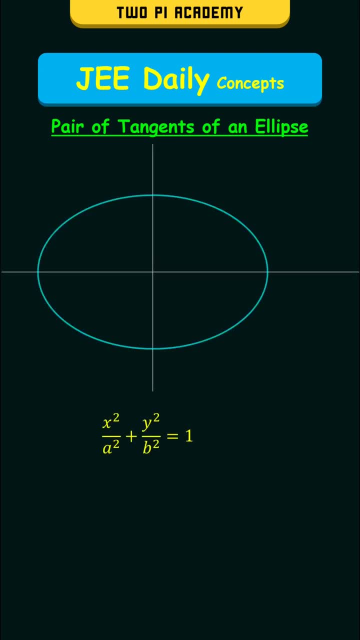 Consider an ellipse with the general equation: x square by a square plus y square by b square is equal to 1, where a is greater than b. And consider a point outside the ellipse, p, Then from this point you can draw two tangents to the ellipse And to find the equations 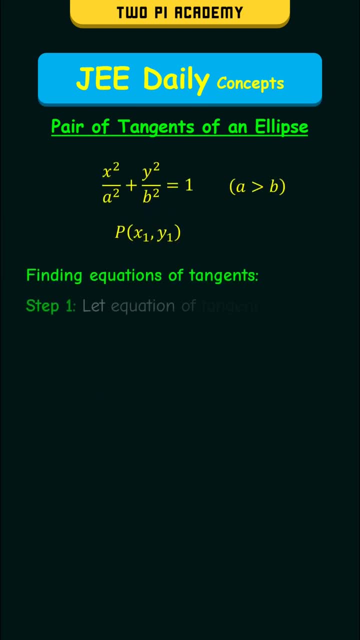 of these tangents, use the following procedure: First, let the equation of the tangent be- y is equal to mx plus or minus square root of a square- into m square plus b square, And then substitute the coordinates x1, y1 in this and solve for the value of m And finally, 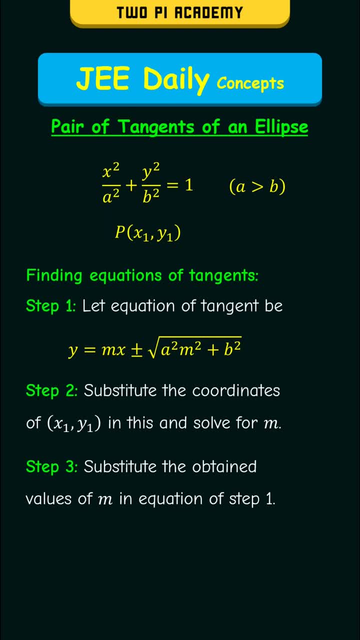 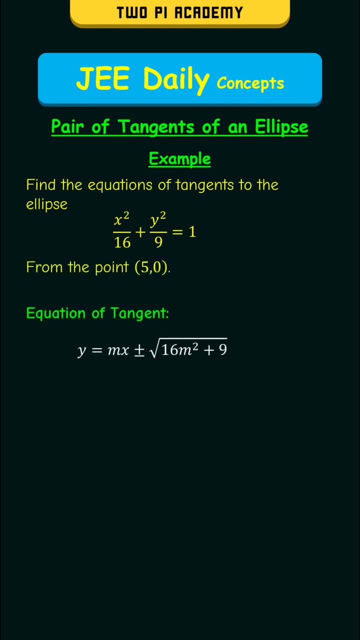 substitute the obtained values of m in the equation of step 1.. For example, let the equation of the ellipse be the following, and let the point be 5 comma 0.. So first let the equation of the tangent be the following, and since this pass through the point 5 comma 0, we can 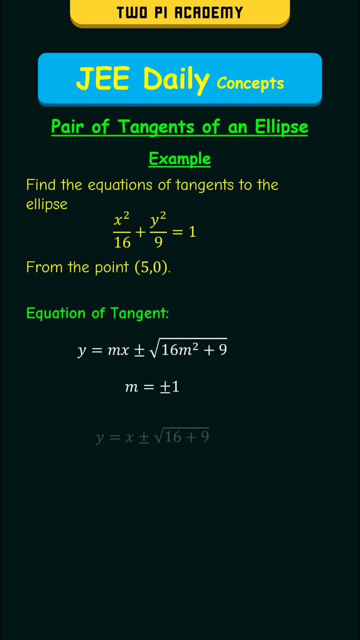 simplify to get m is equal to plus or minus 1.. We then substitute this in the equation of the tangent and since this tangent pass through 5 comma 0, we can get its equations as the following: Please subscribe to channel to not miss any future uploads. And this is: